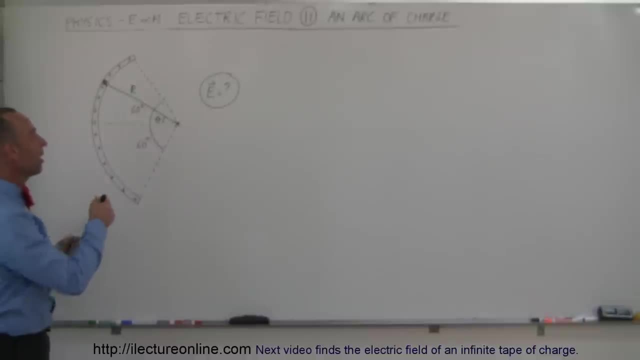 Welcome to Electro-Online. and now we're going to try to find the electric field of a piece of a circle that is charged by positive charge. We call that an arc of charge, And in this particular case, notice that the arc subtends an angle, a total angle of 120 degrees. so 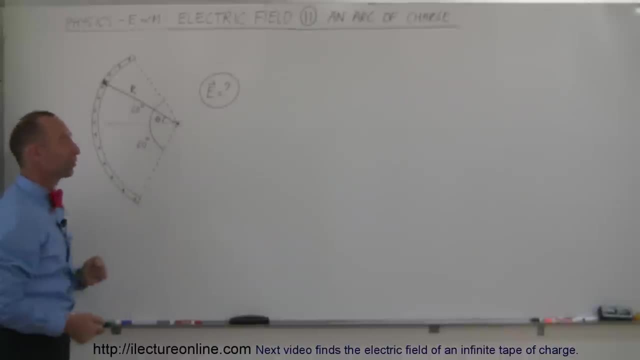 it's about one-third, not about exactly one-third of a circle. The radius is r, and so the charge always resides exactly the distance of r away from the point that we're interested in. Now let's take a small little segment over here and let's call that a small amount of dq, and so 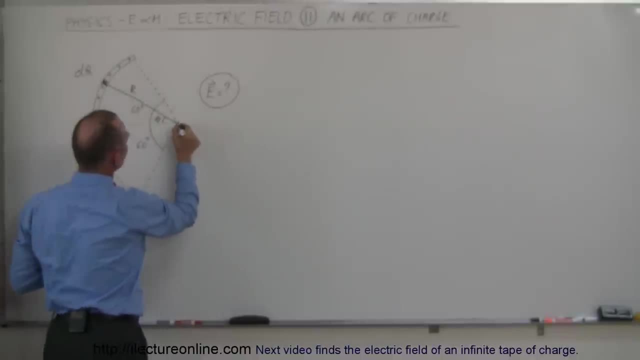 therefore, the electric field at this location, caused by the small amount of dq, is going to be a small amount of dE, And that dE is going to be equal to k times dq divided by r squared r, of course, being the radius of that circular arc. Now notice that on this dE, it's going to have a. 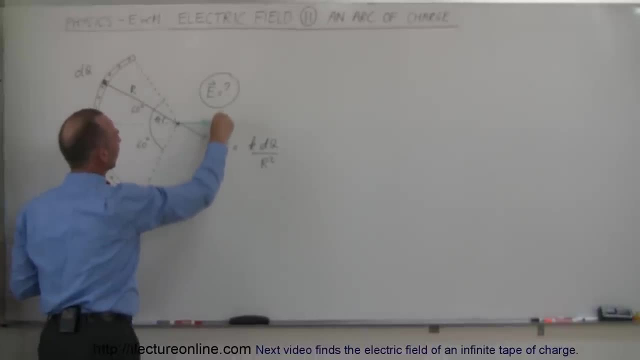 horizontal and a horizontal angle. So that's going to be a horizontal angle And that's going to be a horizontal angle, And that's going to have a horizontal angle And that's going to have a vertical component. There's going to be a dE in the x-direction and a dE in the y-direction, And 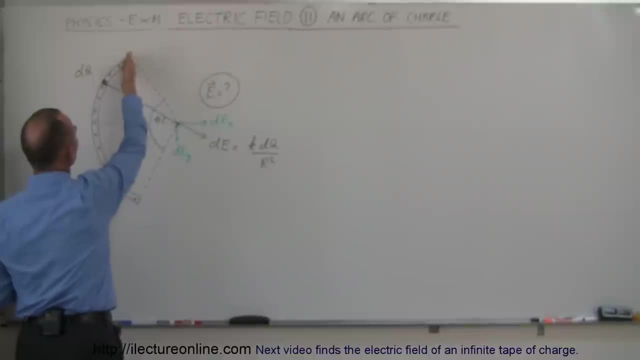 what we know about the vertical components is that all the segments on the top half of the arc will have a vertical component, dEy in the negative direction, and all the segments at the bottom half of the arc will have a vertical component in a positive direction. And 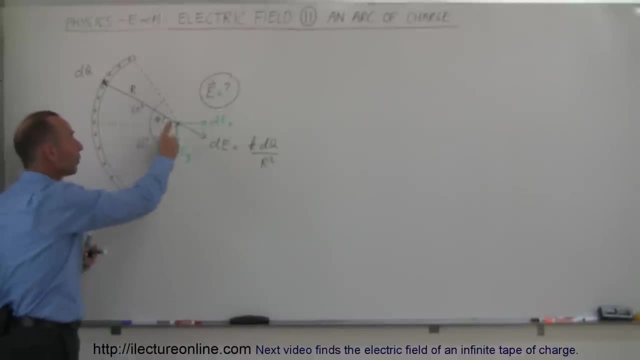 because of symmetry, they will cancel each other out, and so we don't have to worry about the vertical components, they simply cancel out. We only have to worry about the horizontal components, the dEx. And, of course, if this angle here is theta, that means that this: 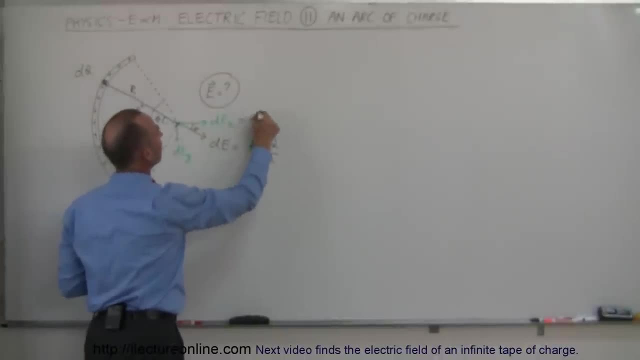 angle here is theta, which means that dEx is equal to dE times the cosine of theta. There's my little angle of theta right there. Alright, now, cosine of theta. what is that equal to? Well, let's see here. It's equal to cosine of theta. I don't think we need to find out. 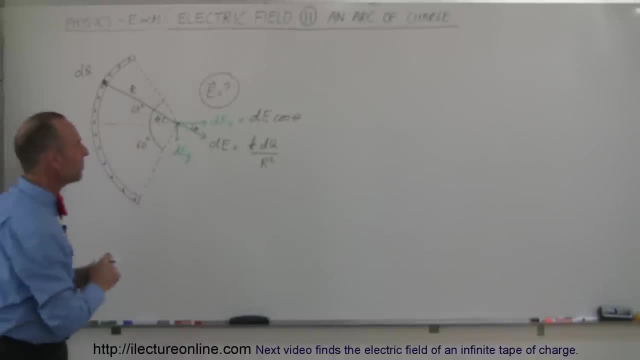 the equivalence, and we'll see in just a moment why that is So. that means that dEx can be written as dE, which is k times dQ over r squared times the cosine of theta. That's dQ, not d theta. so we've got to be careful here. Alright, now how much is dQ? how much charge is that? Well, let's see. here We have. 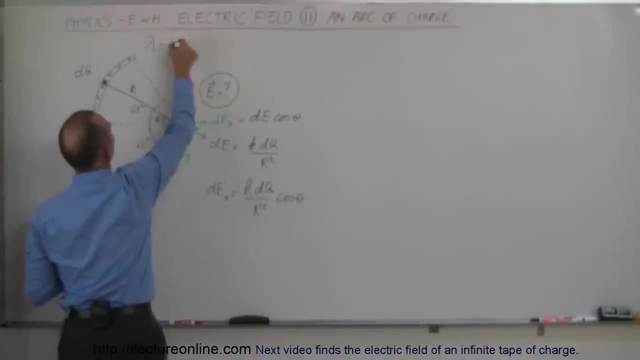 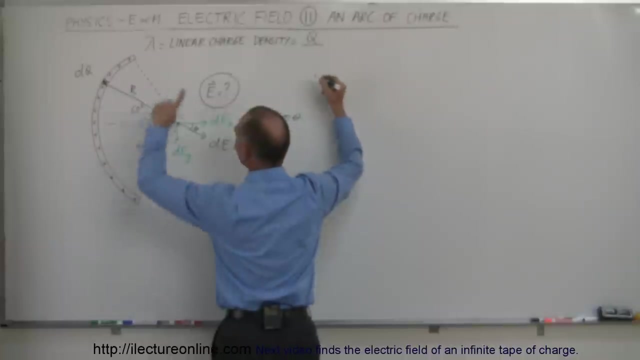 a linear charge density. let's call it lambda. lambda is equal to the linear charge density, which would be equal to the total charge placed on the arch divided by the length of the arch, and that would be one third the circumference of the circle, which is two one. 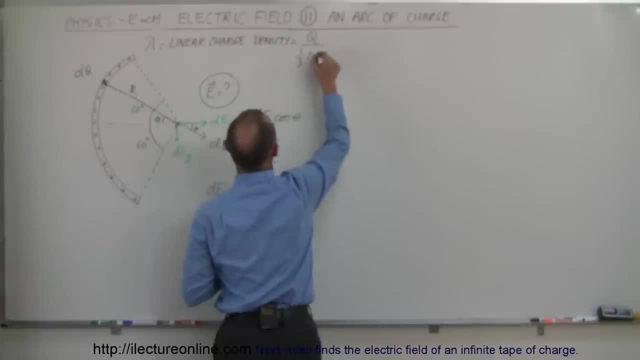 third, i wrote one half, but i meant one third, one third times two pi times the radius, which means three q divided by two pi r is the linear charge density, that's assuming we place the charge q on this arc structure right here and then to find dq, so dq is going to be equal to the linear. 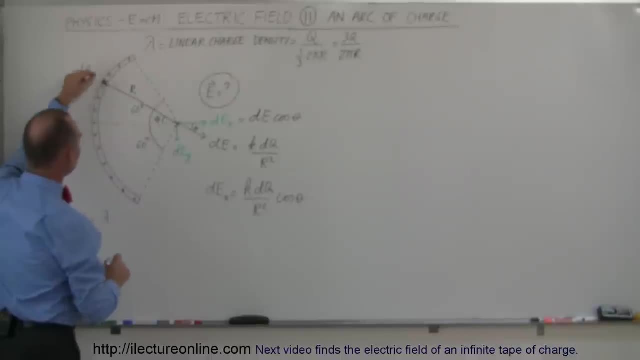 charge, density times, the arc length, and the arc length is going to be a ds, and remember a small segment of arc length, let's see here that subtends an angle, a small angle of d theta. so this would be d theta, and so ds can be written as r d. 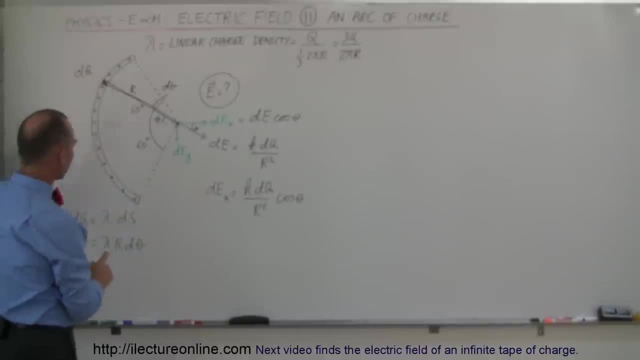 theta. so the dq on this little segment can be written as the linear charge density times r d theta, which represents a small little arc length, ds. so that can go into the equation. so we can write d: e in the x direction is equal to k. instead of dq we're going to write lambda r times d theta. 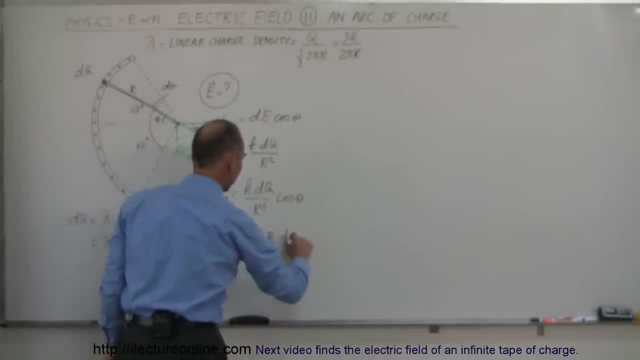 so lambda r times d theta times. the cosine of theta divided by r squared, and then notice that this r will count as d theta. and then we're going to write: lambda r times d theta. times d theta dot r. now to find the total electric field. all we have to do is integrate all the way from this end. 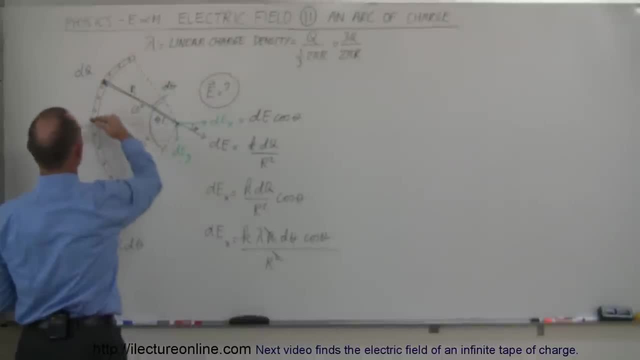 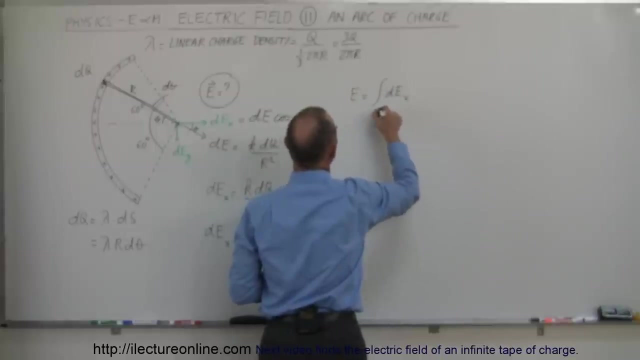 all the way down to this end right there, or we can do halfway. we go from zero to to theta equal sixty degrees, and then double it because of course the symmetry right there. so to find the total electric field e, we have to sum up all the little d e, x's and if we're going to integrate from zero, 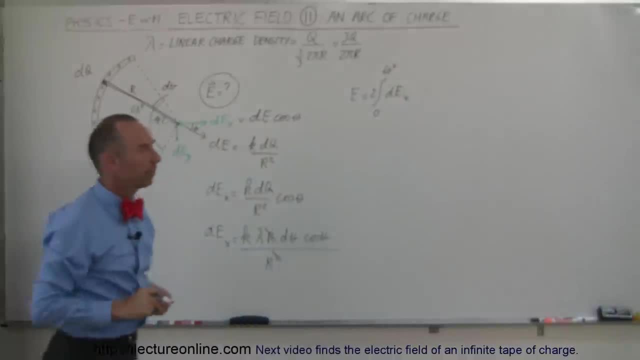 to sixty degrees. we're going to do it twice because there's a symmetry here. so it would be this times 2, and that would be integrating this right here. so that would be equal to 2 times the integral from theta. equals 0 to theta. 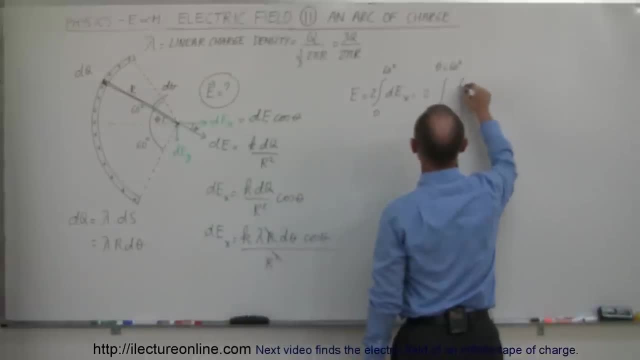 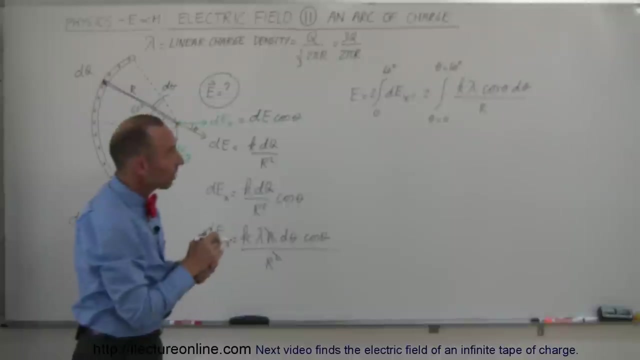 equals 60 degrees of k, linear charge density times the cosine of theta, cosine of theta d theta, all divided by r. Now notice: in this particular case r is a constant, k is a constant, lambda is a constant that can come all out of the integral sine. so we have 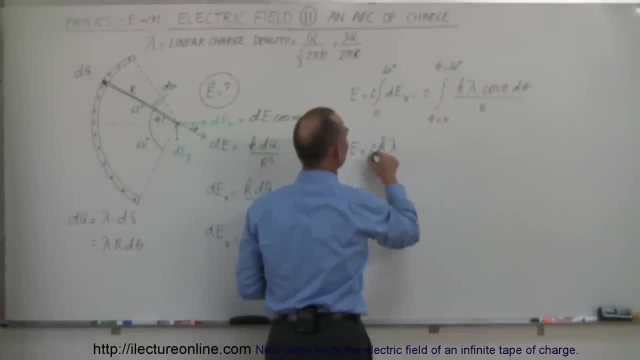 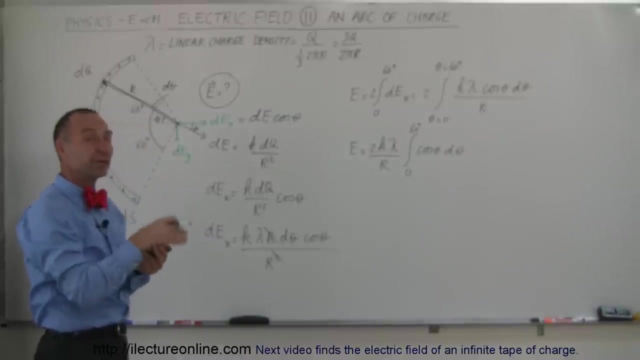 e is equal to 2k lambda divided by r times the integral from 0 to 60 degrees of the cosine of theta, d, theta Alright, and that is fairly easy to integrate. We know that the derivative of the sine is the cosine, so that means the integral of the cosine is d sine. so this: 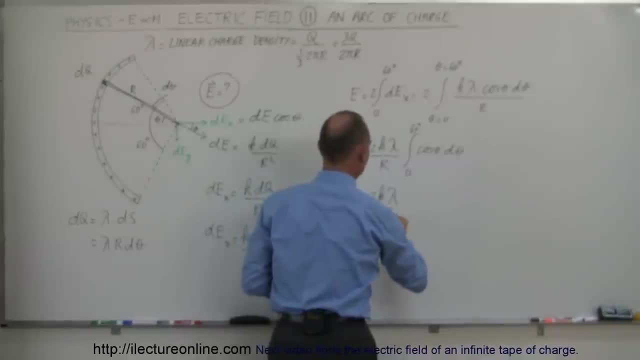 is equal to 2k lambda over r times the sine of theta evaluated from 0 to 60 degrees. Alright, when we plug in the limits, what do we get? This is equal to 2k lambda divided by r times the sine of. 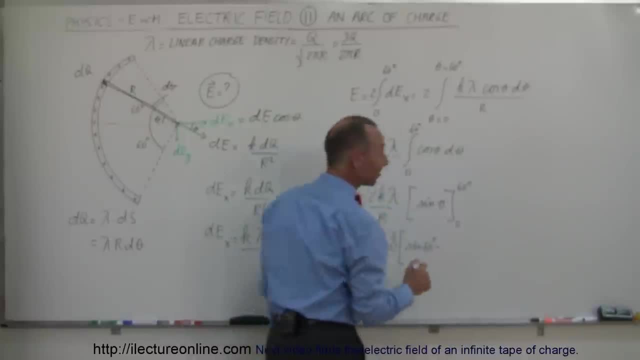 60 degrees minus the sine of 0 degrees. Now the sine of 0 is 0, so we can just plug in the 0 right there. And the sine of 60 degrees is the square root of 3 over 2, so that's. 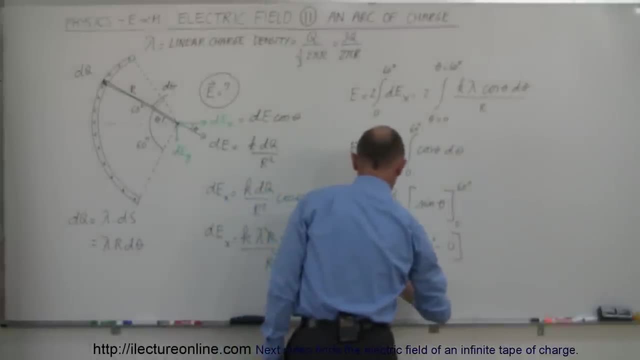 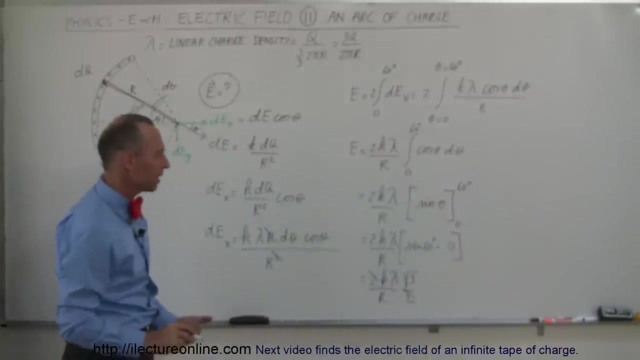 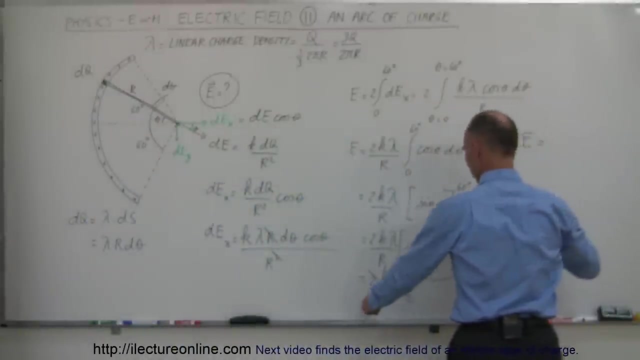 equal to 2k lambda over r times the square root of 3 over 2.. Now these two cancel out. now we're left with the square root of 3 times k lambda over r. So finally, over here we can write that the electric field strength is equal to the square root of 3 times k lambda. 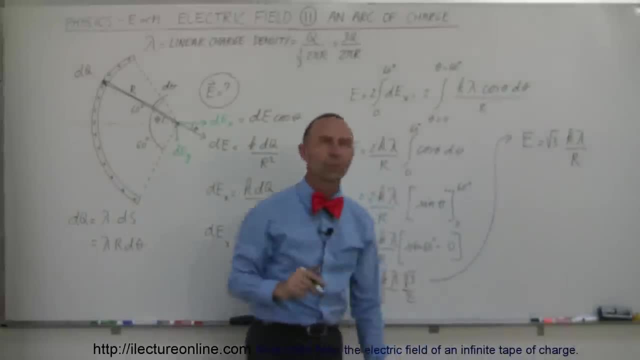 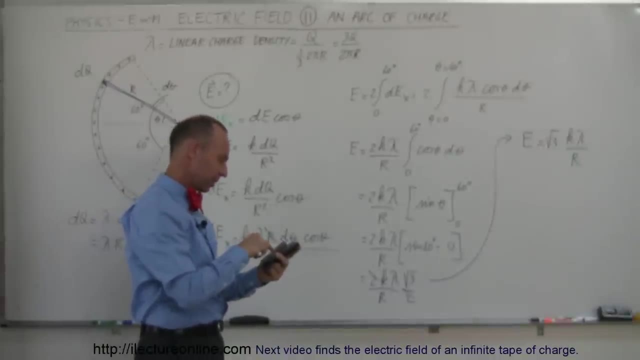 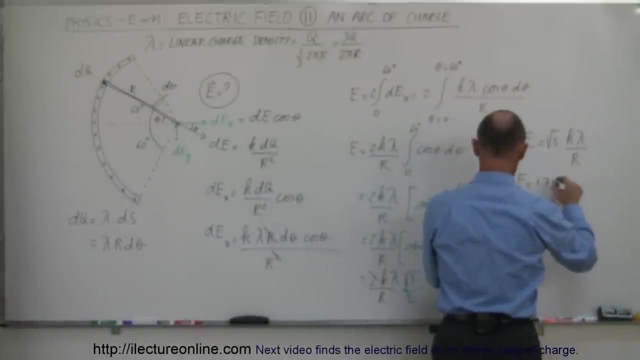 over r And of course the square root of 3 is 1 point. I have to figure that out. Ah, always forget what that is. Take the square root and we get 1 point 1 point 7, 3.. So we can write this: the electric field strength is equal to 1 point 7, 3 k lambda. 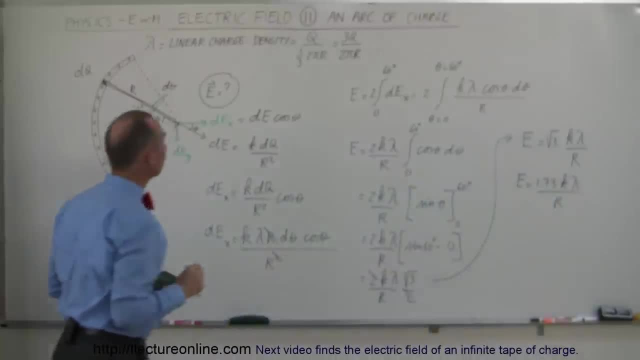 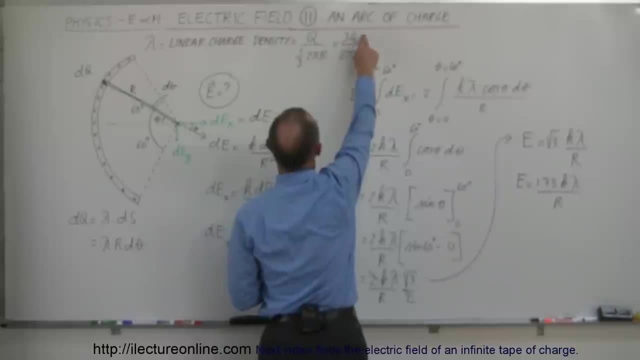 over r. Now we could, we could replace the linear charge density which we have over here by what it's equal to: 3k over 2 pi r. so if we want to do that, we get e is. 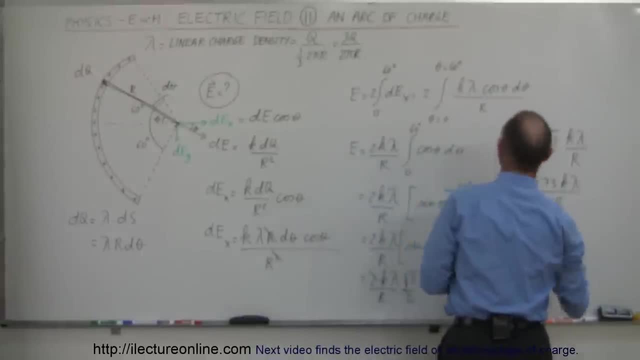 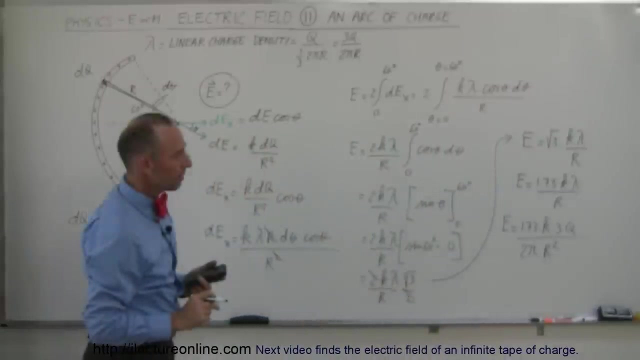 equal to 1.73, or we could have left it as square root of 3, doesn't matter. times k, times lambda, which we can now write as 3 times q divided by 2, pi r times r. that makes it r squared. All right, and now we can just kind of simplify things a little bit, so we: 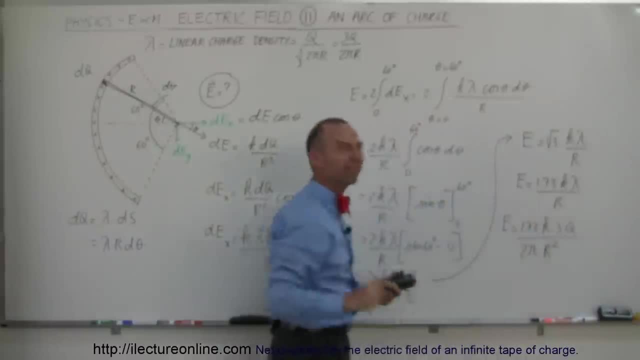 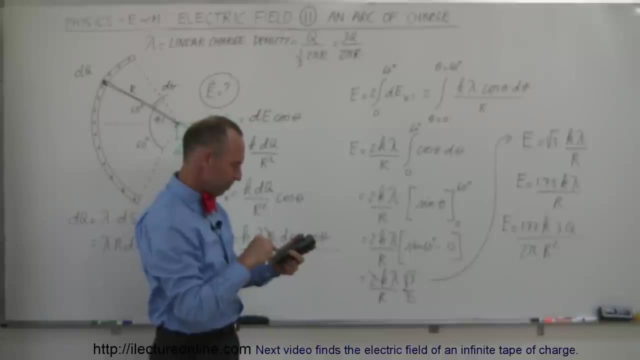 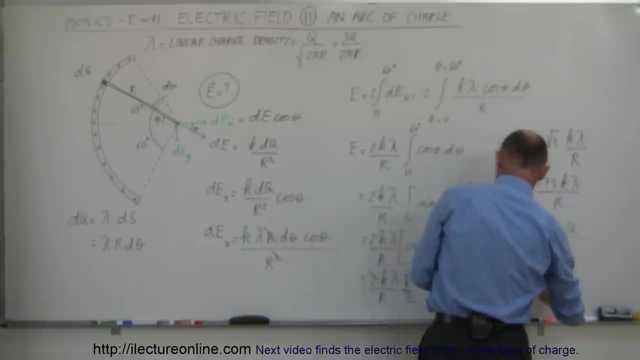 take 1.73 times 3 divided by 2, divided by pi, and let's see what that equals to. So 1.73 times 3 divided by 2, divided by pi, okay, so now we get. e is equal to 0.827 kq over r. 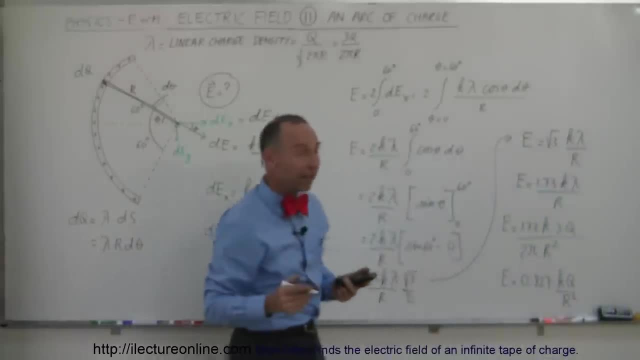 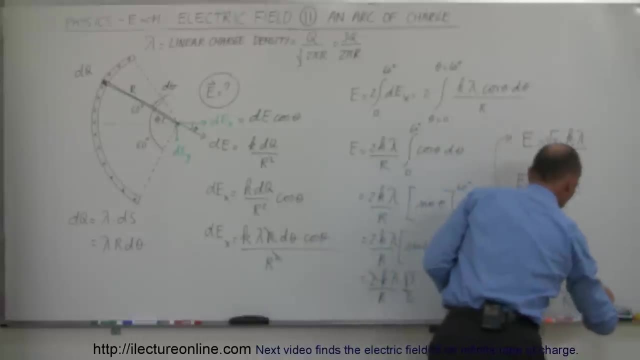 squared, and that's probably the best form to leave it at Now. also, let's see here: if we want to turn that into a vector, notice that it'll be to the right, so we can make that into a vector quantity with the unit vector near. 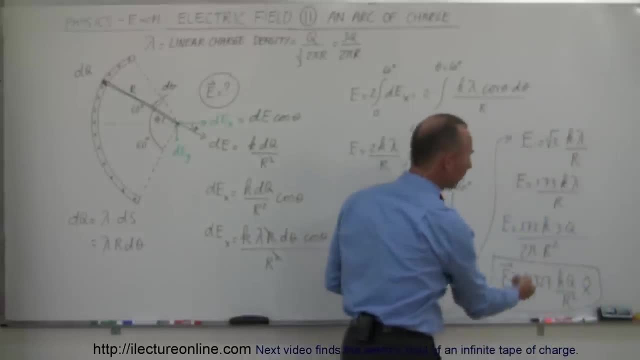 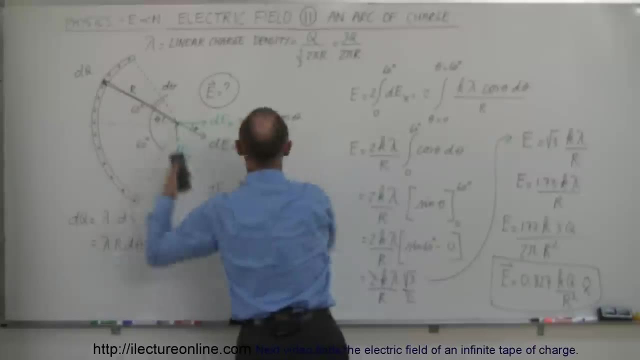 Next direction. and there you go. Now notice that this is in your typical format for the electric field: kq divided by r squared. r squared, of course, that's the distance squared to the point of interest, and times 0.827, that's a constant added to that equation. 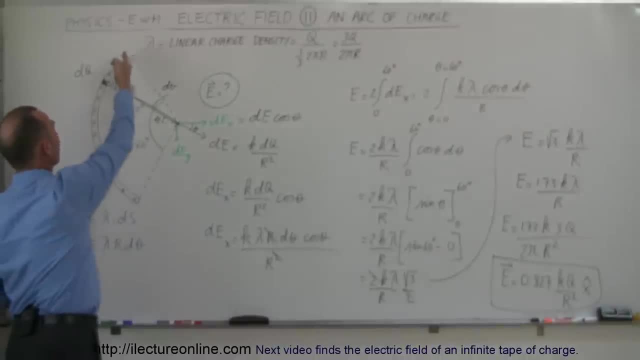 and that is the what we call electric field, due to a arc of charge and, of course, the point being at the center of that arc. If it's not at the center of the arc, it's further away. that becomes a much more difficult problem. 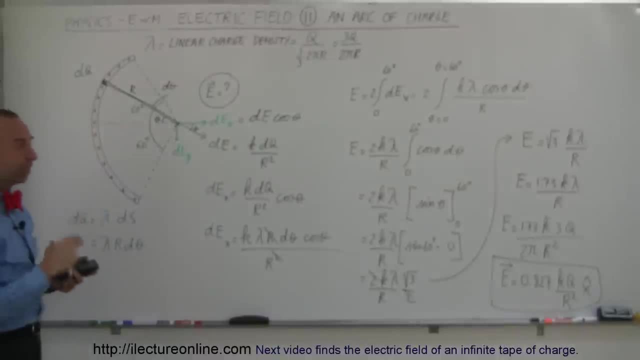 And that's for a different kind of video. All right, so that's how we do this one.